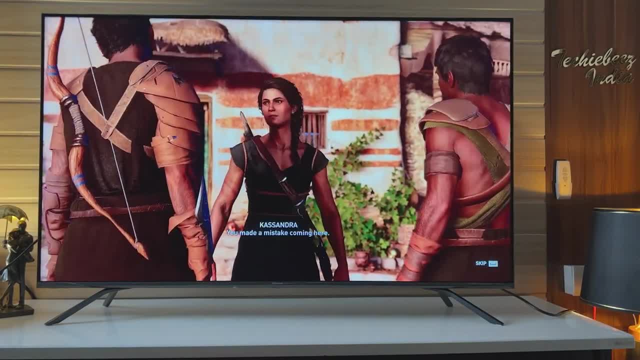 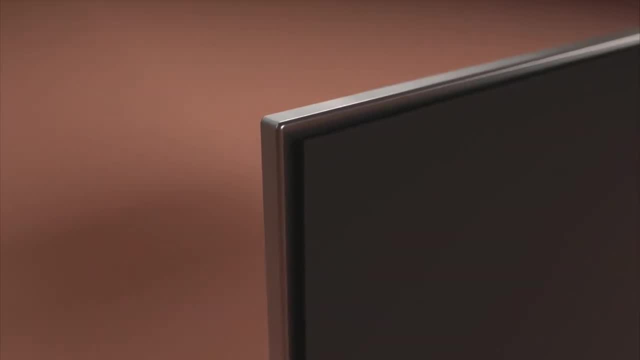 the low input latency, Allowing quick and responsive gameplay. the U6 runs on Google TV, providing an effortless way to find and enjoy your favorite content. With voice search, a wide selection of apps and personalized recommendations, it enhances the streaming experience. The TV also features: 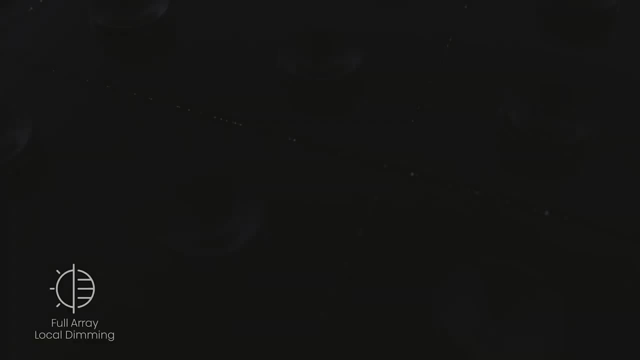 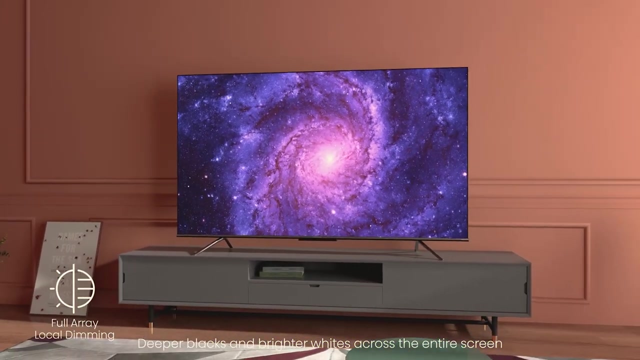 built-in Chromecast for easy content streaming from your devices and a voice remote for convenient control. In addition to its image quality and smart TV capabilities, the U6 includes a built-in soundbar that delivers decent audio quality. It supports Dolby Vision and Atmos, two advanced 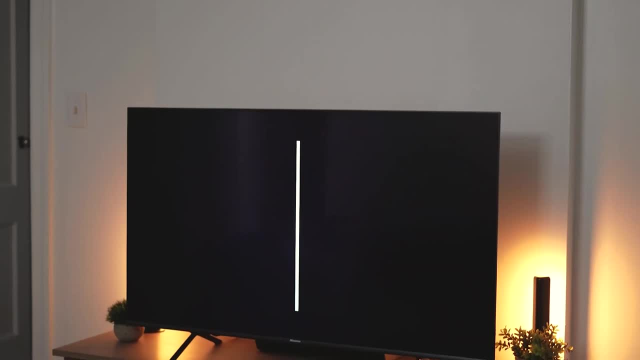 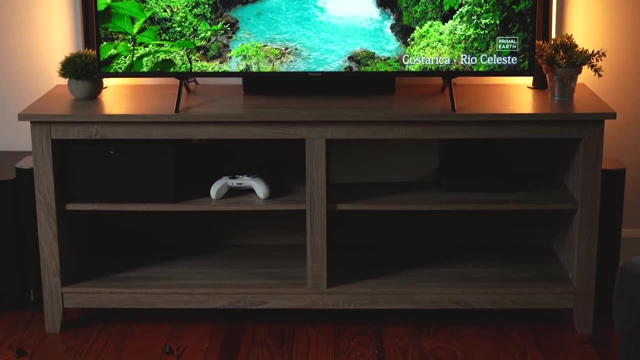 HDR formats. The TV is equipped with multiple ports, including 4 HDMI, 2, USB and an Ethernet port. The Hisense U6 comes in 55-inch or 65-inch screen sizes with a 4K Ultra HD resolution. Its ULED panel. 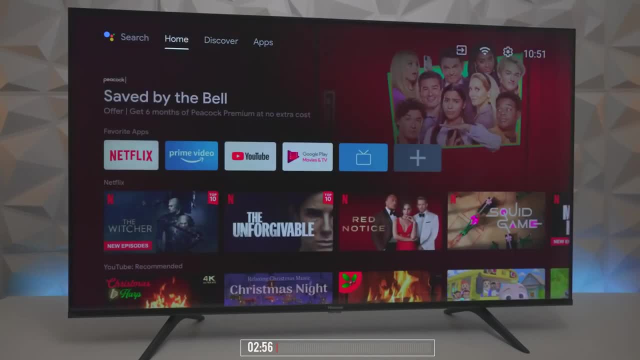 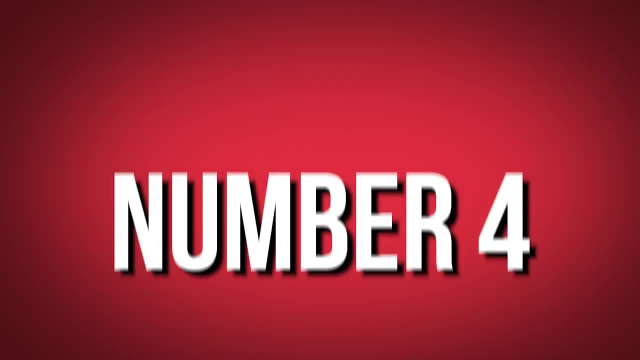 ensures stunning visuals, and the low input latency of 12.5 milliseconds enhances gaming performance. The TV also supports variable refresh rate- VRR, minimizing screen tearing. Number 4.. Sony X90J, With its stunning 4K resolution and advanced technologies like 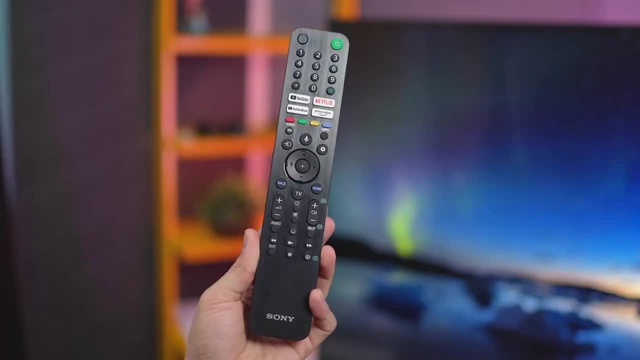 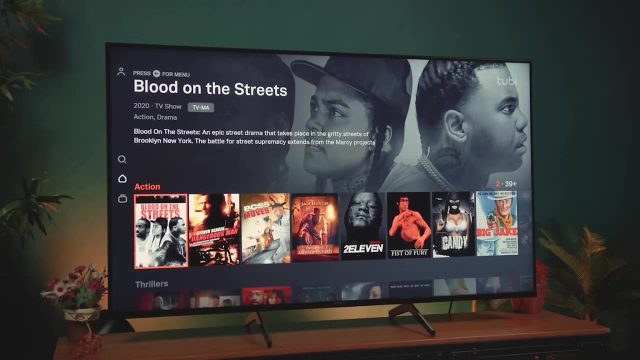 full-array LED backlighting. the U6 is a great choice for a TV. The U6 is a great choice for a TV. The X90J offers an unparalleled immersive viewing experience. The design of the Sony X90J is sleek and modern, with slim bezels and a premium-looking stand. Setting it up is 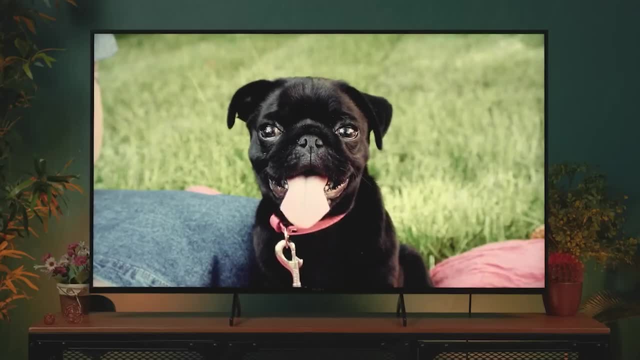 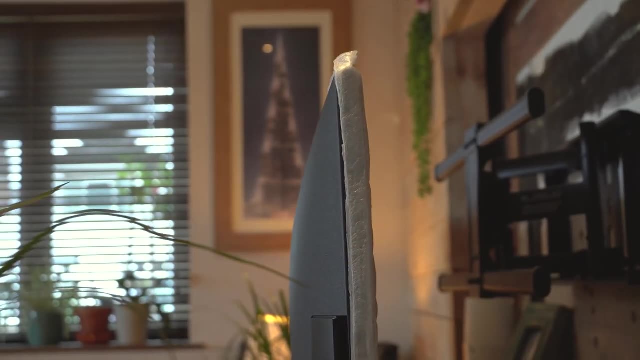 straightforward thanks to clear instructions and an intuitive interface that guides you through the process quickly. When it comes to image quality, the X90J truly impresses. The 4K resolution delivers sharp and clear visuals with vibrant and vivid colors that pop. 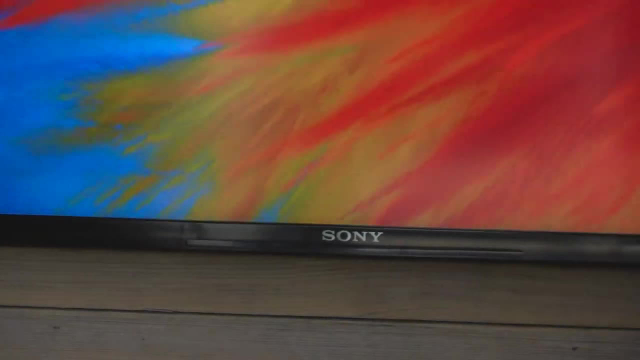 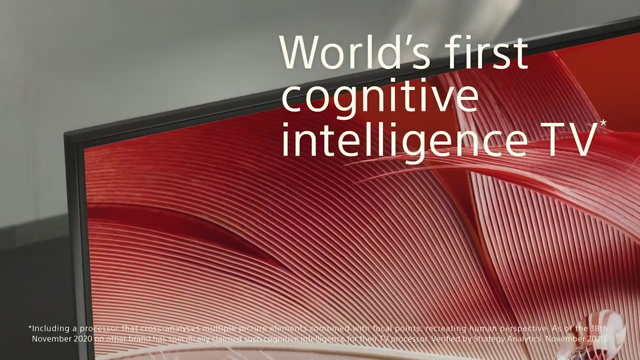 The full-array LED backlighting ensures even light distribution, minimizing glare and enhancing image quality from any seating position. HDR support on the X90J is excellent, with brighter highlights and less noisy shadows. Whether you're watching movies, TV shows or playing games, the X90J offers an immersive 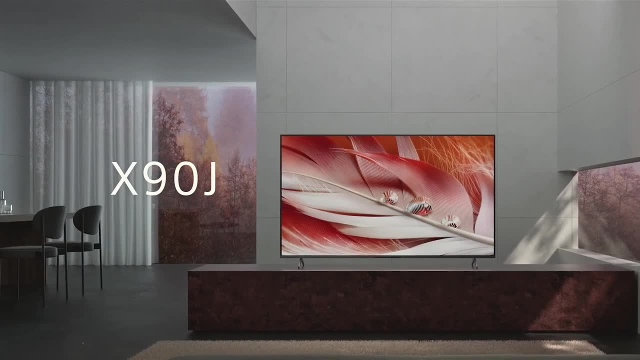 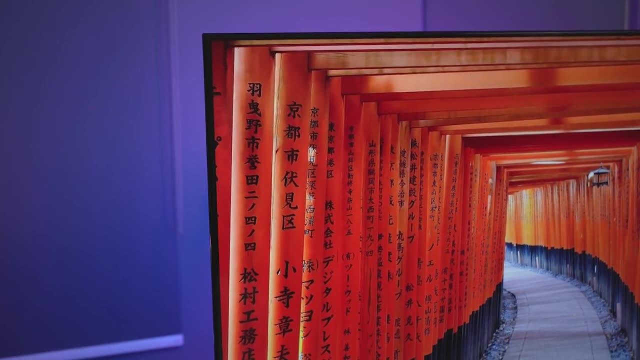 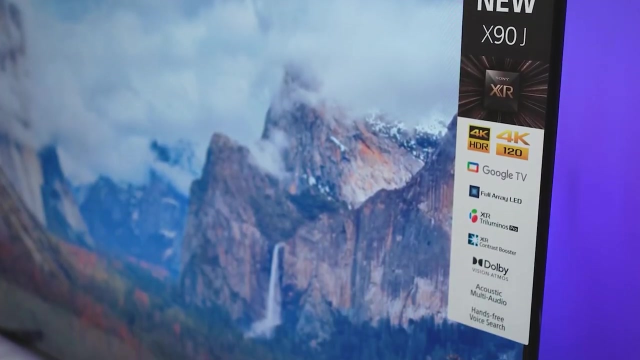 visual experience. Sound quality is also impressive, with support for Dolby Atmos, delivering a rich and immersive audio experience that brings your entertainment to life. While it may not replace a dedicated home theater system, the built-in speakers are more than sufficient for most users. The X90J's smart TV features are top-notch. 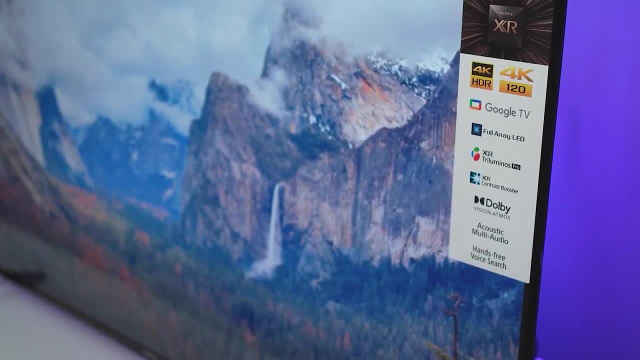 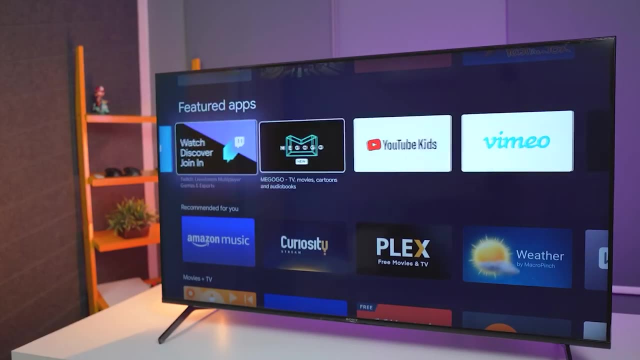 with built-in Wi-Fi and support for popular streaming services like Netflix and Amazon Prime Video, Accessing your favorite content is seamless. The interface is user-friendly, with a quick and responsive menu for easy navigation. Connectivity options on the X90J are abundant. 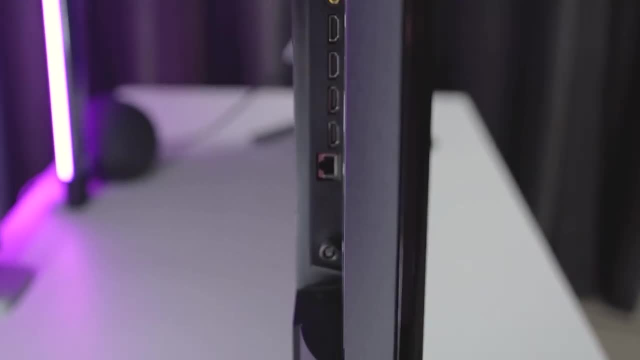 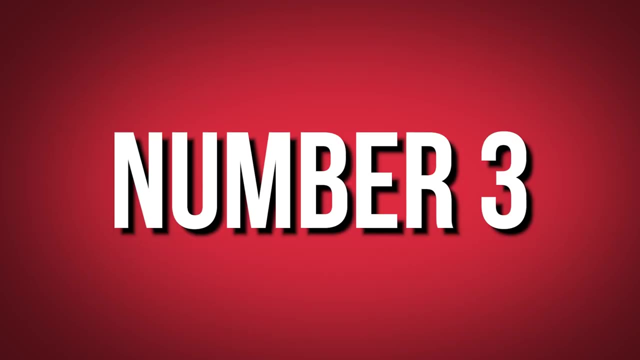 including HDMI, USB, Ethernet and Bluetooth. This allows for easy connection of external devices like gaming consoles and soundbars, enhancing your entertainment experience. Number 3. LG OLED C1. With outstanding contrast, a wide color gamut and low input latency, it's a great choice for. 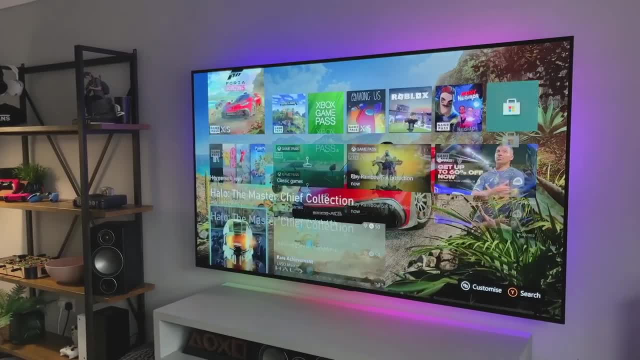 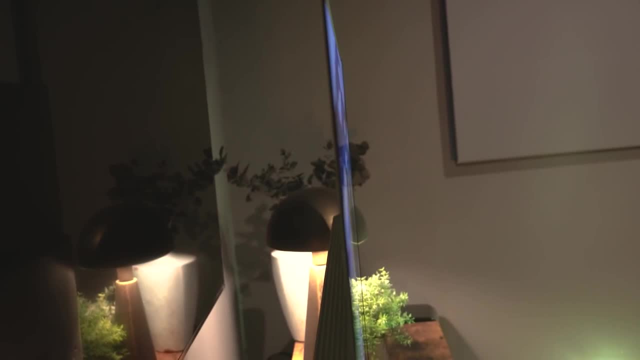 movie enthusiasts and gamers. The C1's image quality is a major selling point. Its OLED panel delivers excellent contrast by individually turning off pixels, resulting in perfect blacks. This is particularly beneficial for dark movies or TV shows, as the blacks are truly black. 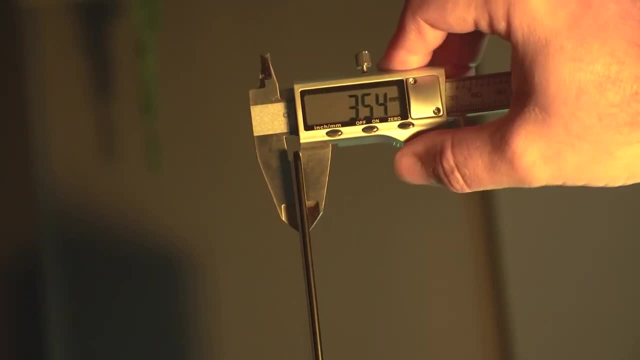 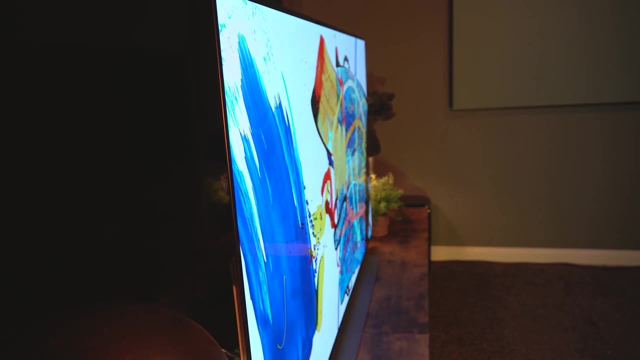 The C1 also offers a wide color gamut, allowing it to reproduce a broader range of colors than most TVs. This is essential for HDR content, as it brings out more details in shadows and highlights. Gaming on the C1 is also impressive The low input latency. 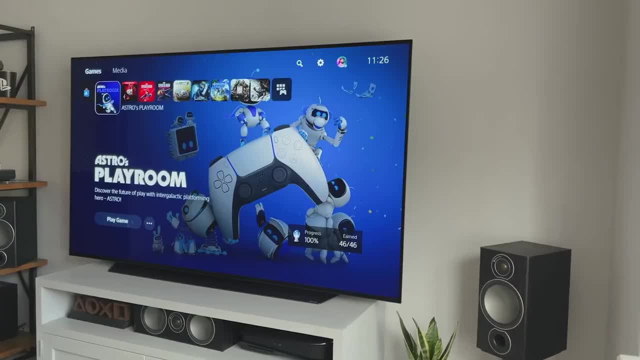 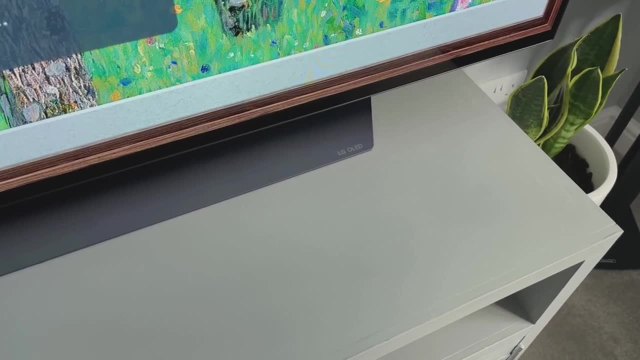 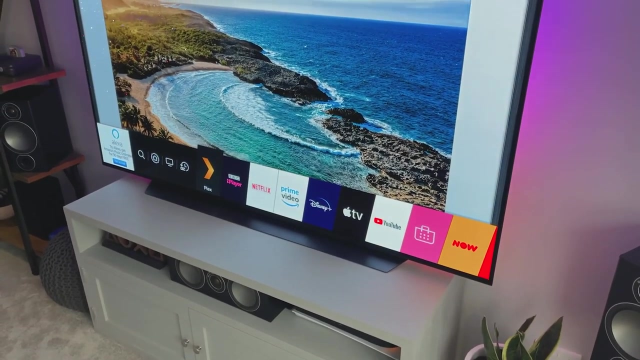 ensures minimal delay between controller input and on-screen action, which is crucial for competitive gaming and quick reactions. Operating on webOS, an intuitive platform, the C1 makes finding and watching favorite content effortless. It offers a wide selection of apps, including popular services like Netflix, Hulu, Amazon, Prime Video and Disney+. 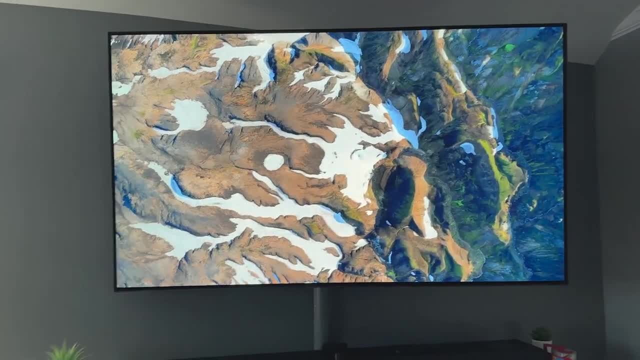 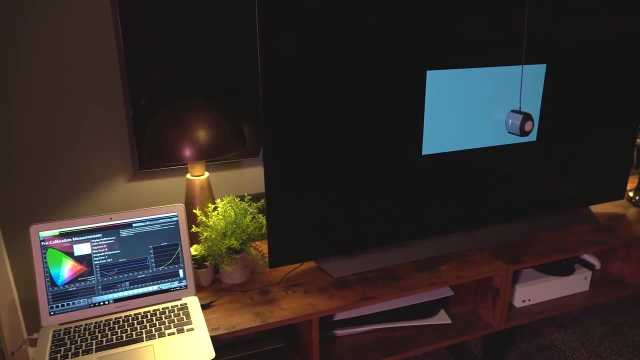 The built-in voice assistant enables convenient control through voice commands. Additionally, the C1 boasts other smart TV features, including built-in Chromecast for seamless content streaming from mobile devices. The included voice remote control enhances user experience, In addition to its image quality and. 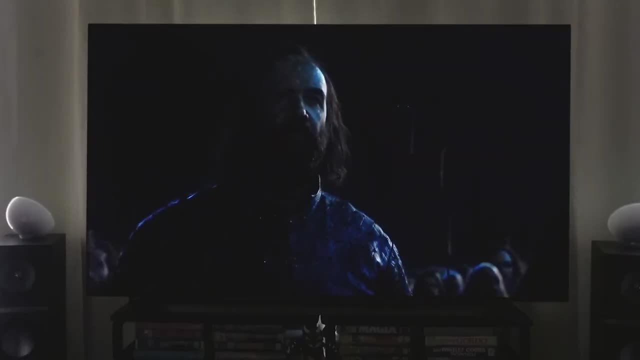 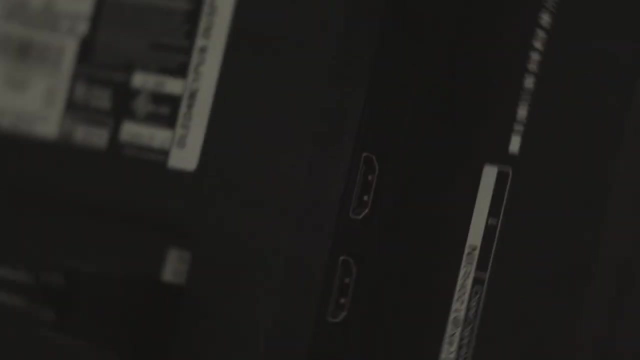 smart TV features. the C1 is well-suited for home theater setups. It includes a built-in soundbar providing decent sound quality, and supports advanced HDR formats like Dolby Vision and Atmos. Multiple ports, including 4 HDMI, 2 USB and an Ethernet port, offer versatile connectivity. 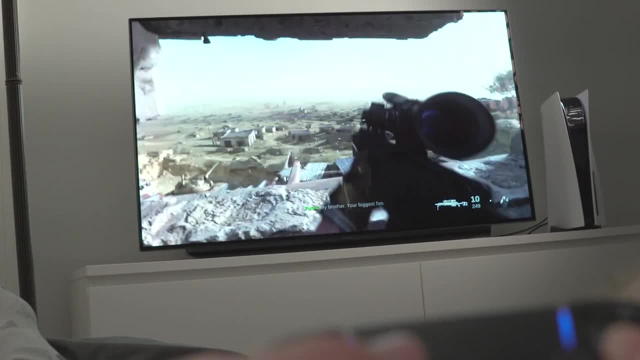 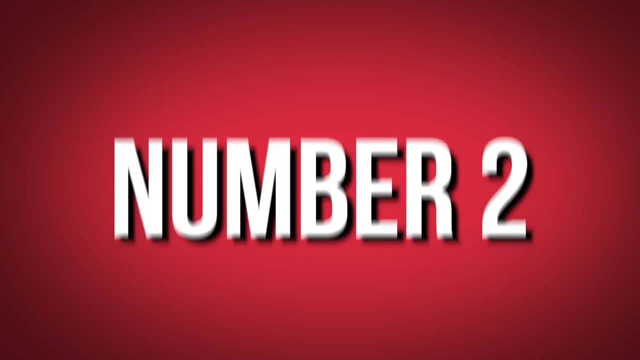 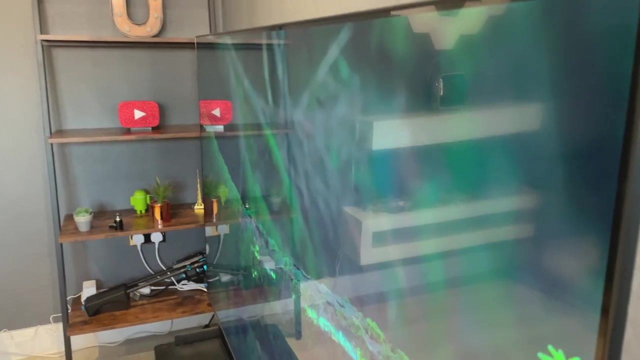 options. Overall, the LG OLED55C1PUB is an excellent value for money. If you're looking for a smart TV, the C1 is a fantastic choice. Number 2. Samsung AU8000. The Samsung AU8000 smart TV is a feature-packed television with excellent performance. that is. 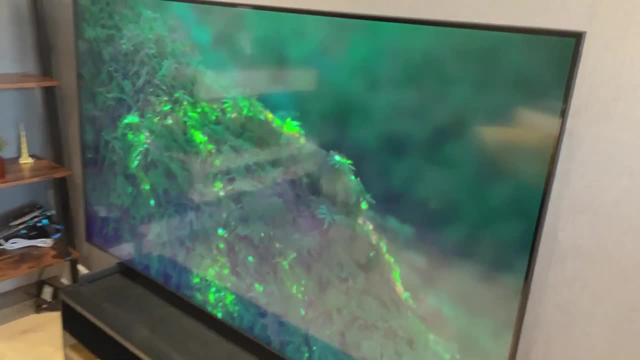 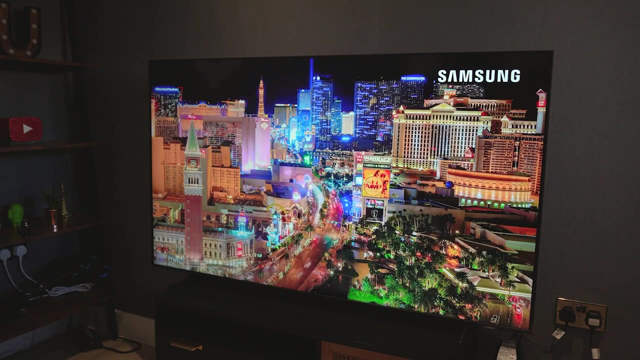 quickly becoming a popular choice for those seeking an affordable yet reliable 4K TV. With its stunning design, advanced technologies and intuitive smart interface, the AU8000 caters to both casual viewers and demanding users. First and foremost, the design of the Samsung. 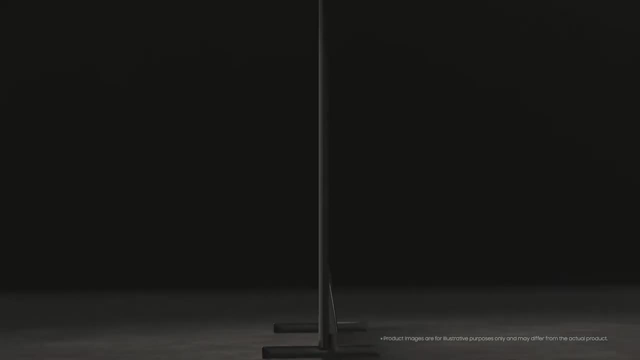 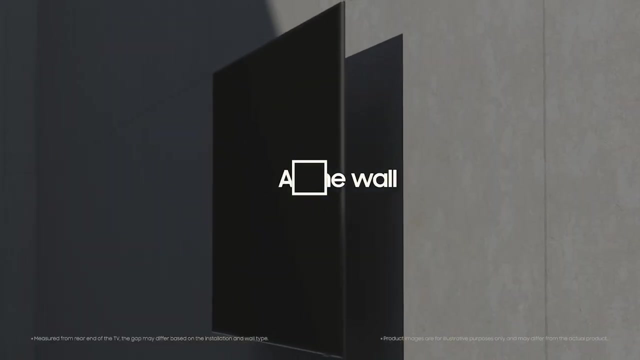 AU8000 is elegant and minimalist, featuring a slim bezel and a sleek body that seamlessly blends with any room decor. The TV is a great choice for those looking for a smart TV. The C1 is a stylish stand that elevates it a few centimeters from the ground, giving it a premium look. The TV 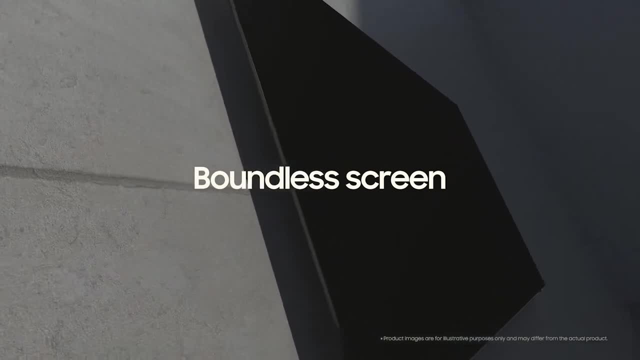 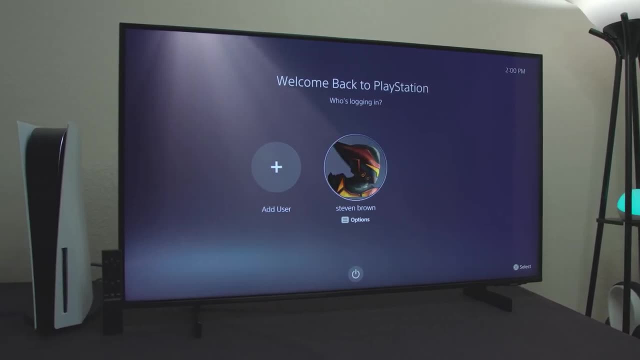 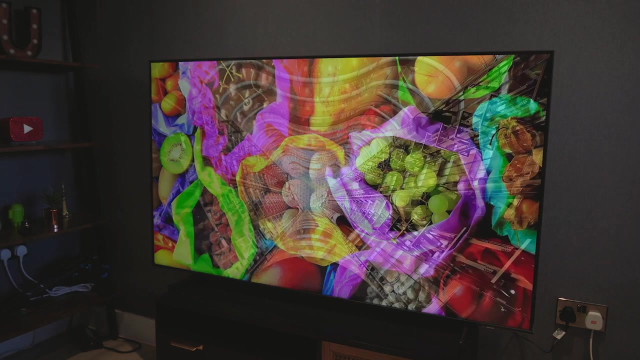 is relatively lightweight and easy to assemble, with clear instructions guiding you through the setup process. The AU8000 displays impressive image quality, with 4K resolution and HDR support that delivers stunning and accurate colors. The screen is bright and offers excellent contrast ratio, while color accuracy is simply breathtaking. Blacks are deep and dark. 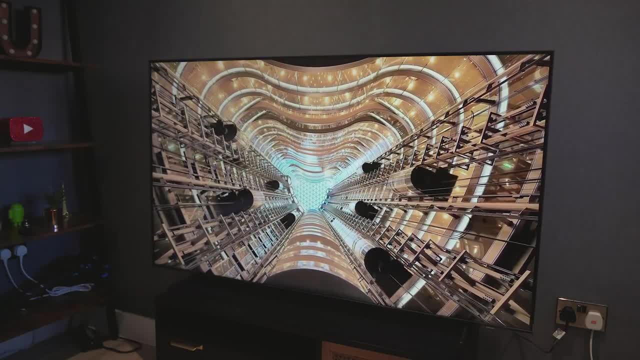 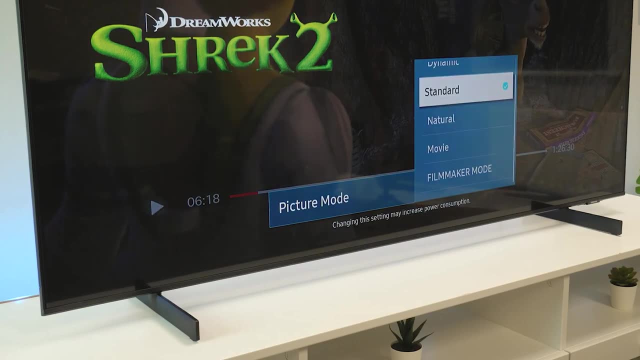 and the brightest highlights are luminous and consistent, creating a truly captivating visual experience. The AU8000 features an advanced crystal 4K processor that enhances non-4K content, such as HD or standard definition, to convert it into 4K. The TV's motion accelerator technology. 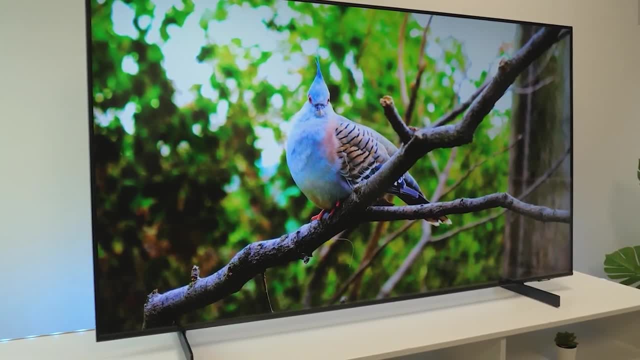 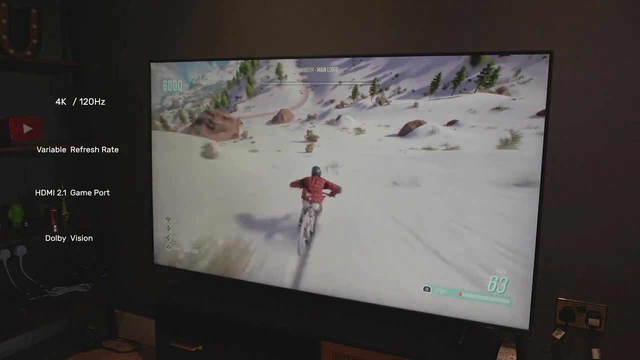 is fantastic. reducing blur and motion drag in fast-paced content like sports or action-packed movies. This feature improves clarity and sharpness compared to other TVs in its class In terms of sound. the Samsung AU8000 is equipped with three built-in speakers that deliver simply. 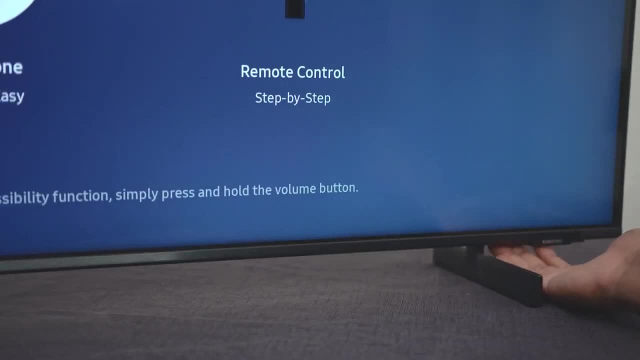 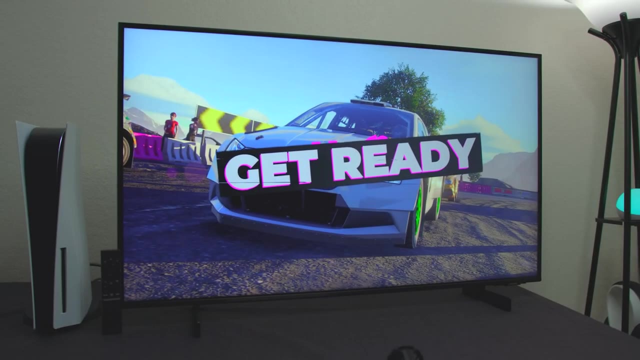 yet quality sound, offering good clarity without being overwhelmingly loud. The TV supports Dolby Audio, enhancing the sound experience by providing a cinematic and immersive feel. While the audio quality may not be mind-blowing, it is more than sufficient to meet the needs of. 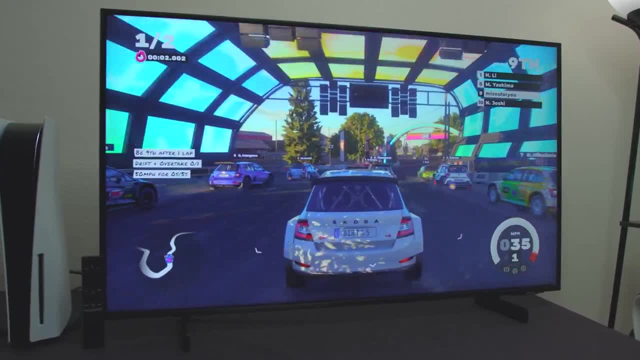 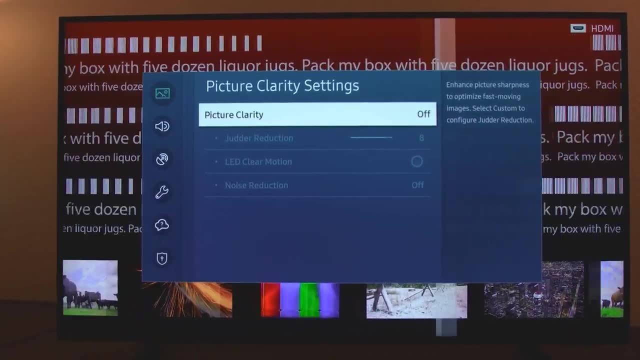 an average user. The smart TV features of the AU8000 are impressive, with the Tizen operating system making navigation a breeze. Users can easily connect the TV to their home Wi-Fi network, allowing them to access their favorite streaming services like Netflix, Prime Video, Hulu. 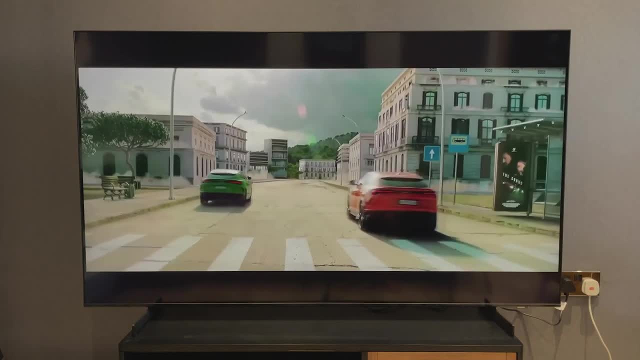 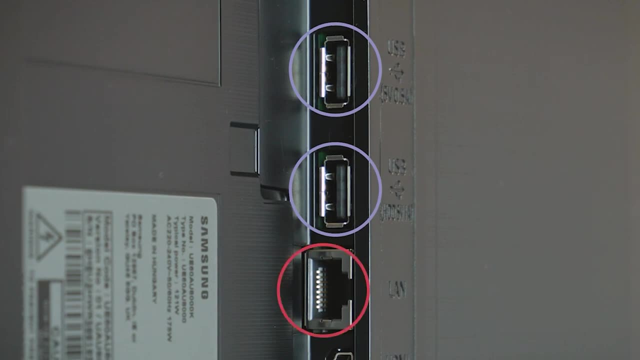 and many others without delays. The unique One Remote feature works seamlessly, enabling the TV to recognize and connect with the TV. The AU8000 features an advanced crystal 4K processor that can connect with other devices such as cables or soundbars. Finally, the Samsung AU8000 offers. 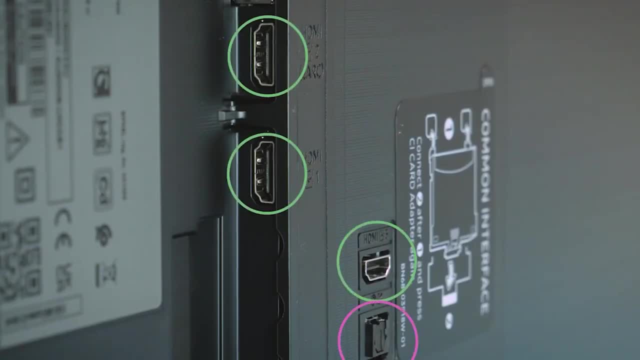 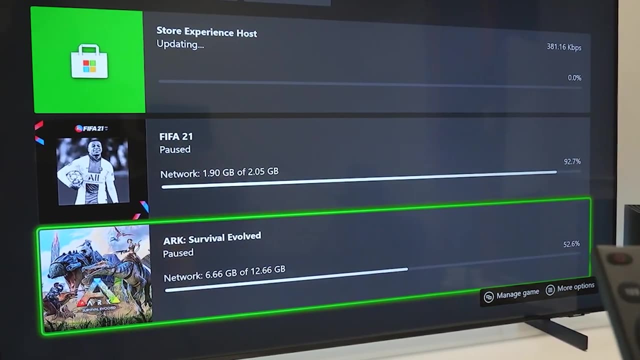 various connectivity options, including Wi-Fi and Bluetooth for wireless connectivity. On the backside, there are three HDMI ports, two USB ports, an Ethernet port, an RF input and an optical audio output. These ports allow users to connect external devices such as gaming consoles. 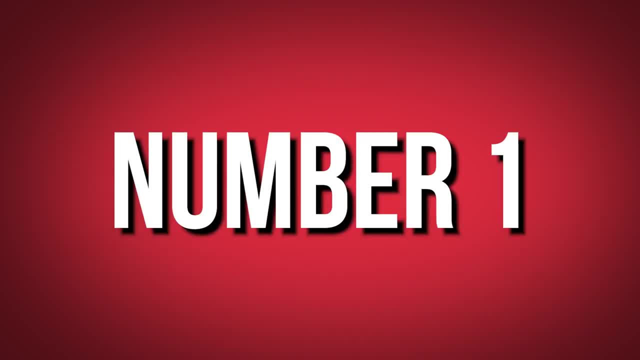 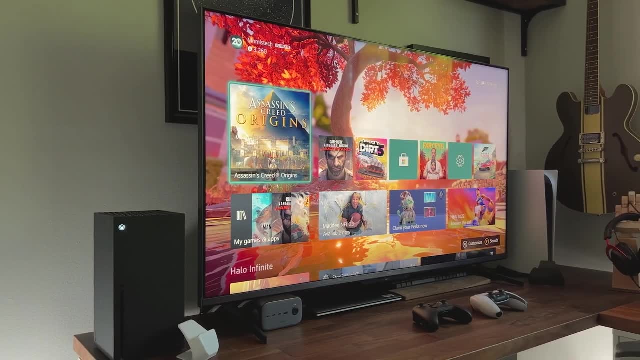 TV decoders, soundbars and external storage devices. Number 1. TCL 4K 6-Series Google TV. The TCL 4K 6-Series Google TV is a QLED 4K television that offers excellent value for money With its outstanding contrast. 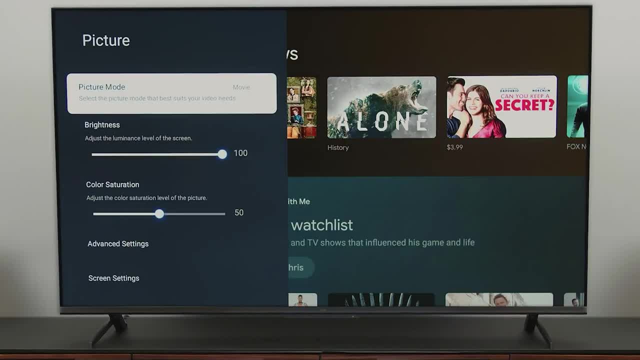 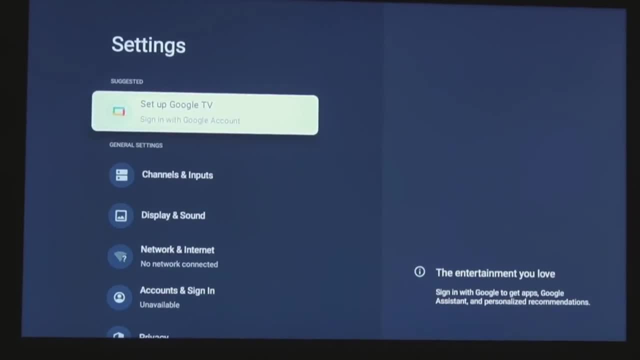 wide color gamut and low input latency, it's a top choice for both movie enthusiasts and gamers. The 6-Series excels in image quality, thanks to its QLED panel that delivers deep blacks and vibrant whites. Watching dark movies or TV shows becomes a captivating experience as the blacks 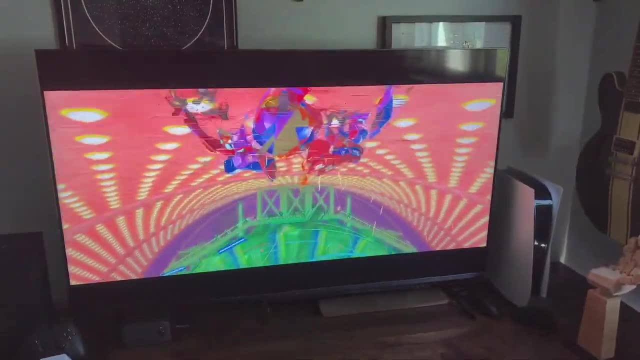 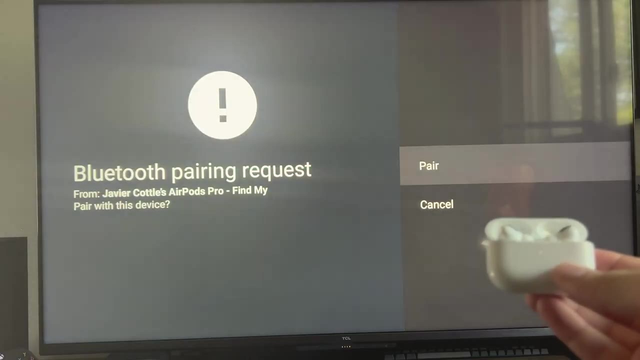 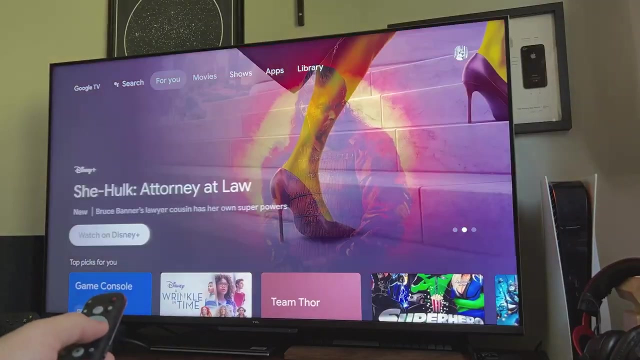 truly appear black, not just dark gray. Moreover, its wide color gamut allows for a greater range of colors compared to most TVs, enhancing the viewing experience of HDR content by revealing intricate details in shadows and highlights. Gaming performance on the 6-Series is impressive thanks to its low input latency, The minimal 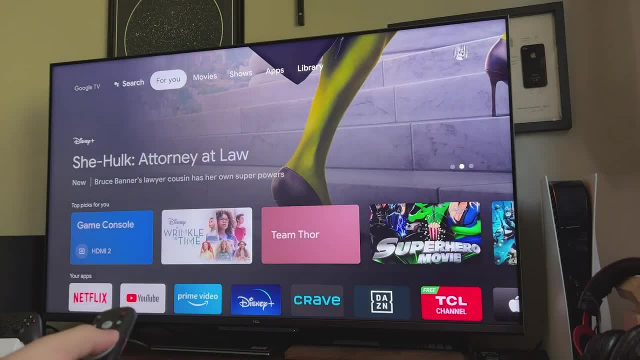 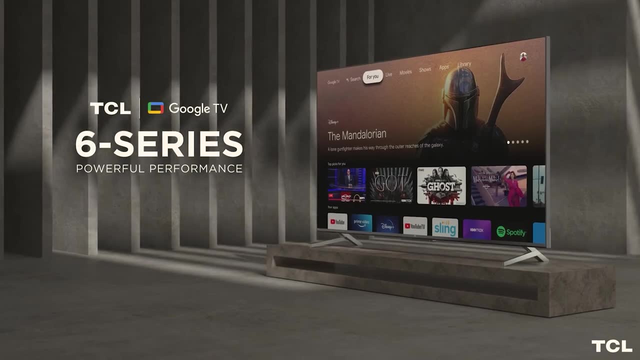 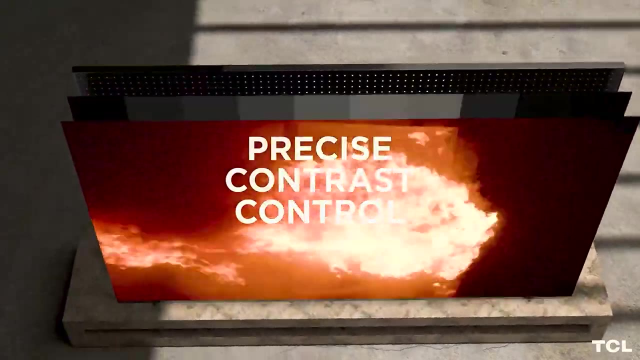 delay between pressing a button on your controller and seeing the action on the screen ensures a seamless gaming experience, particularly for competitive play, where swift reactions are crucial. Running on Google TV, the 6-Series boasts an easy-to-use operating system that simplifies content discovery and viewing, With a vast library of applications, including popular 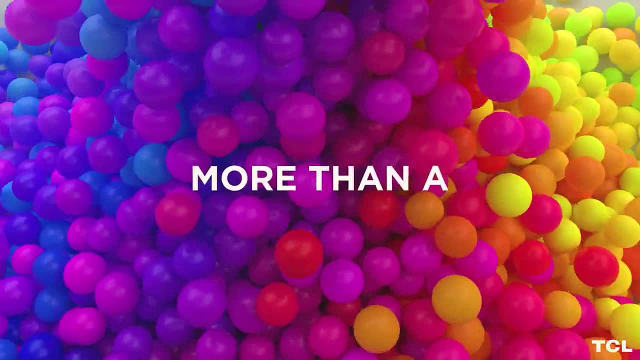 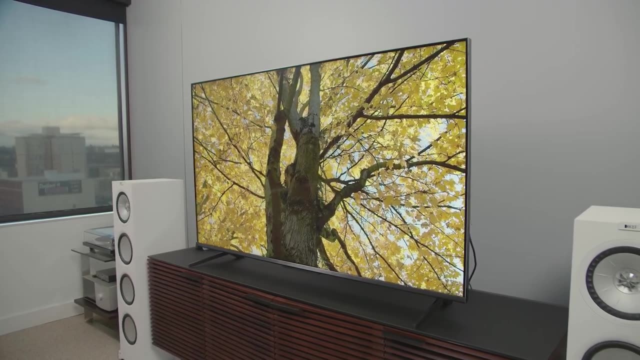 platforms like Netflix, Hulu, Amazon Prime Video and Google Play. the 6-Series is a perfect example of a smart TV that can be easily controlled. Additionally, the built-in voice assistant allows for convenient TV control using voice commands. The 6-Series also offers a range of smart TV features, including built-in Chromecast for 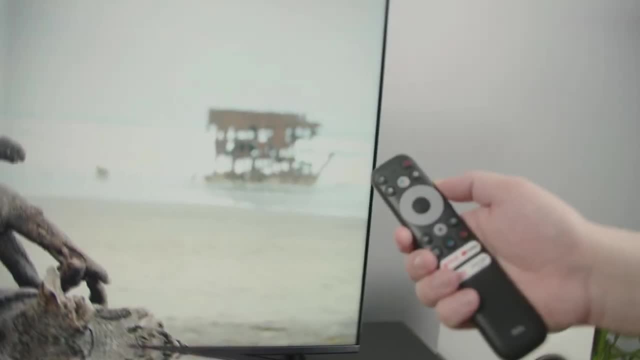 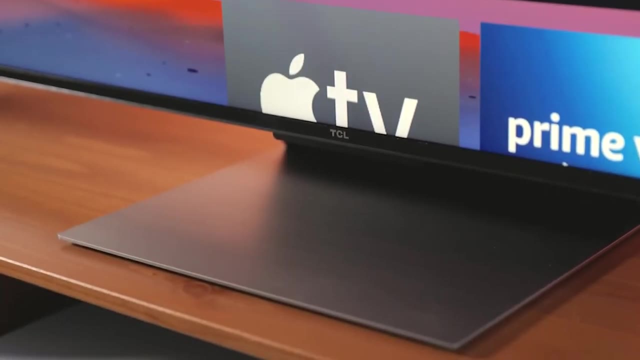 seamless content streaming from your mobile devices to the TV. The voice remote control further enhances the user experience by providing effortless control using voice commands. It features a built-in soundbar that delivers decent audio quality and supports advanced HDR formats like Dolby Vision and Atmos. With multiple portals, the 6-Series is a great choice for 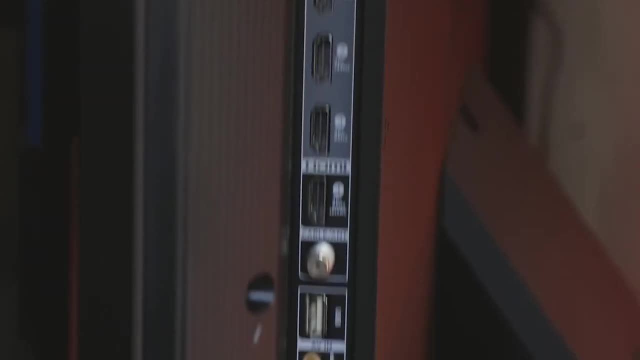 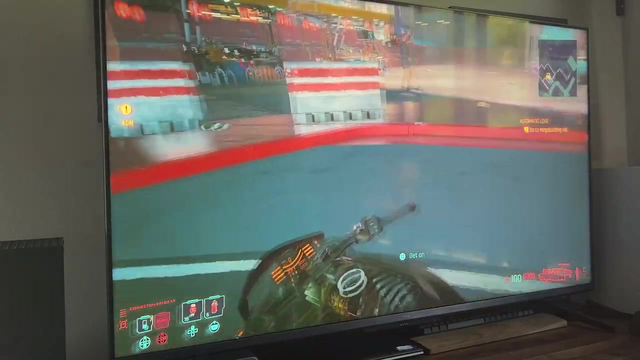 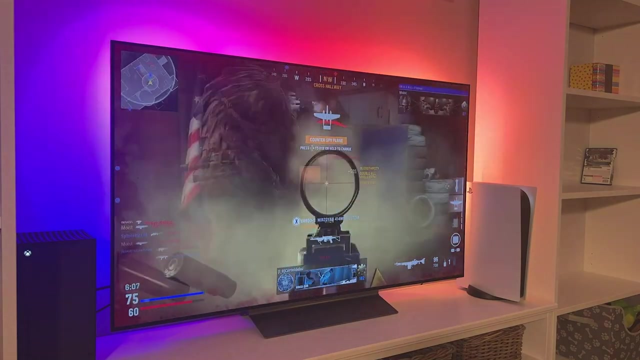 gaming. The 6-Series also comes with 4 HDMI ports, 2 USB ports and an Ethernet port. Connectivity options are abundant, With screen size options of 55 or 65 inches, a 4K Ultra HD resolution of 3840 by 2160 pixels and a low input latency of 12.5 milliseconds. the TCL 4K 6-Series- Google.